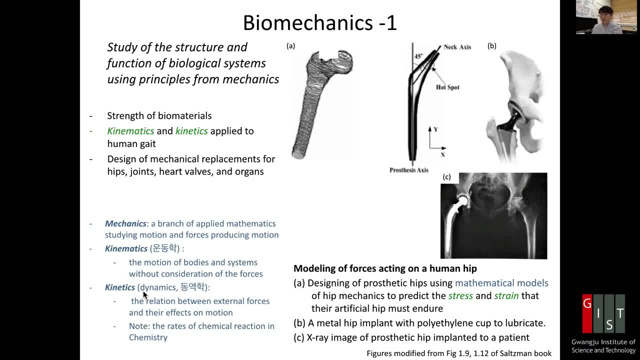 kinetics, or we call it as a dynamics, So that dynamics. now we start to consider the forces, the relation between external forces and their effect on motion. Of course this derives from the famous Newton's law of motion. Just to note to you that in chemistry, 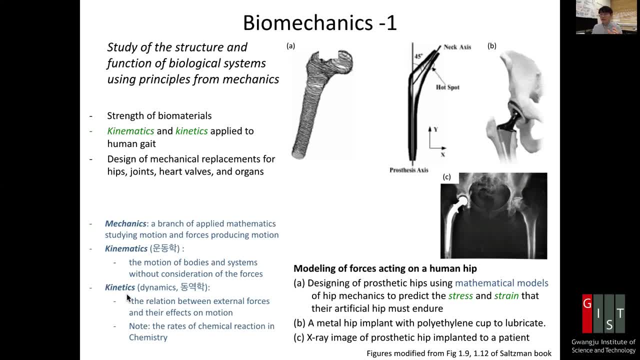 chemical kinetics. that kinetics actually means the rate of chemical reaction in chemistry. So to model, to design this artificial joint that replaces a human hip, what would be necessary To design the prosthetic hips? we use mathematical models of hip mechanics to predict the stress and strain that these artificial hips must endure. 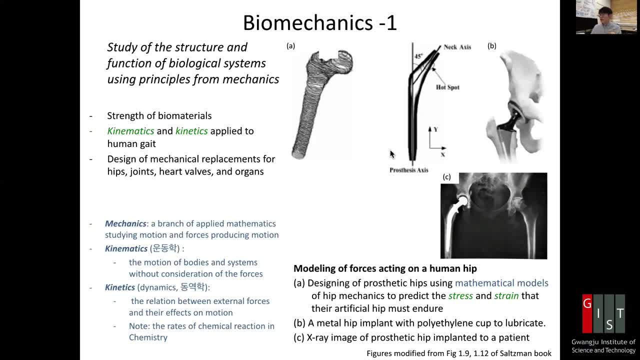 So that mechanical consideration is very important. And also you can see, with these kinetics the perfused joint, be that this hip joint, which is a ball and socket joint, and there there are considerations. so a metal hip implant with polyethylene cup to lubricate it's. 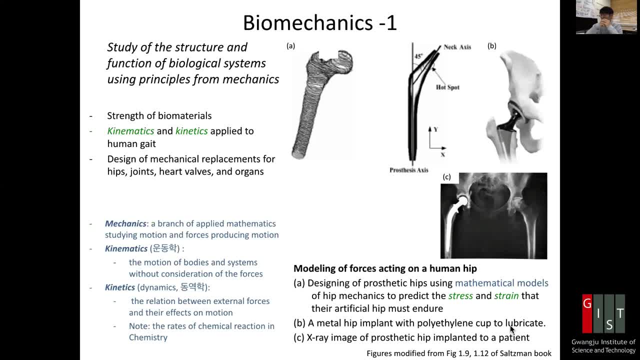 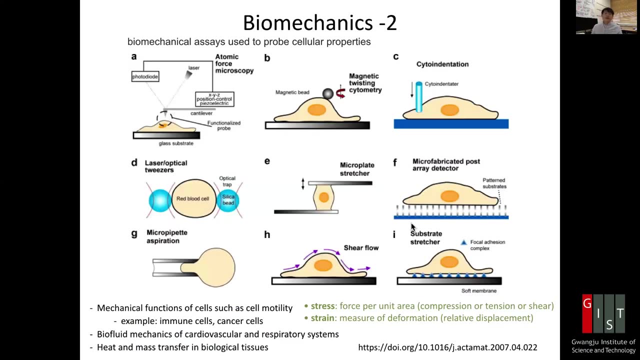 not only mechanical, but also our lubrication has to be under consideration. so this x-ray images shows what is going on after this replacement. so when we talk about mechanics, we can consider maybe big scale. however, our body, down to the tissue and cell and even inside subcellular organelle and 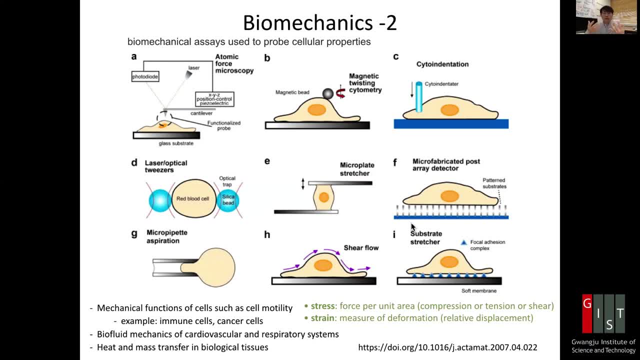 that molecular level there are forces and motions involved. so even when we talk about biomechanics, that can get down to the cellular level too, you so here. I brought some examples of biomechanical assays used to probe cellular properties. so even we want to know the mechanical properties of the 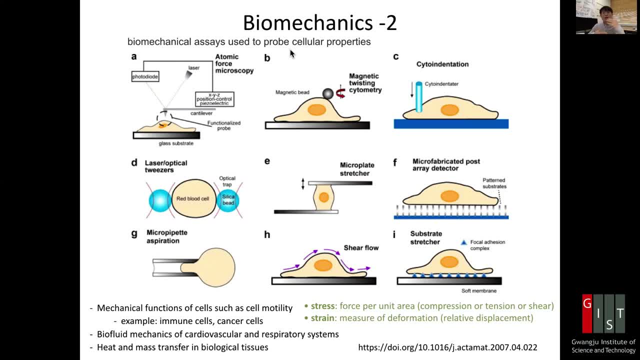 cell and that complicated interaction with the environment is can be very important in some situations. so, for example, mechanical functions of cells, such as cell motility. so we know that when there are outside inserts, such as bacterial attack or viral infection, our immune cells are very, very motile. this motility could be very important for our immune. 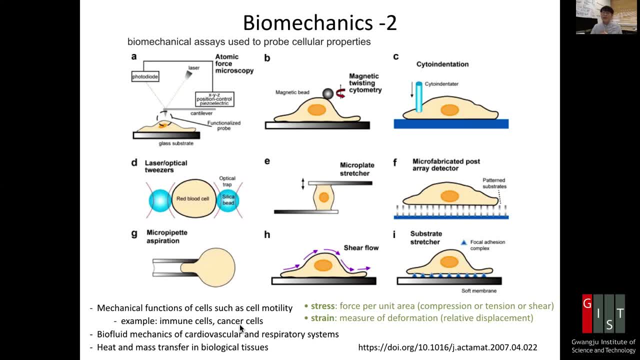 function also. another example is a cancer cell. so if cancer cells grow in one site, in a primary position, it may not be that light threatening. the problem of much of cancer death is from so-called cancelled metastases, which required a cancer cell to grow, becoming invasive, and crawl out of its initial position to 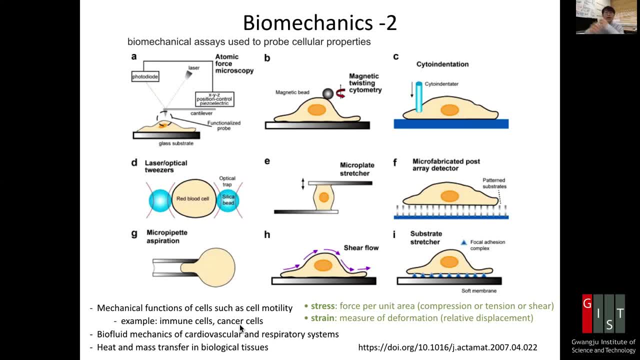 move to distant place where they explode, which become very difficult to treat, for this process requires cancer cell to move and that in that involves a mechanical function. Another example of biomechanics is biofluid mechanics of cardiovascular and respiratory system. So in some way our body especially 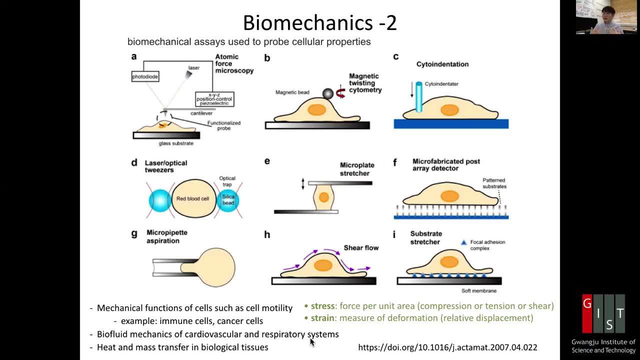 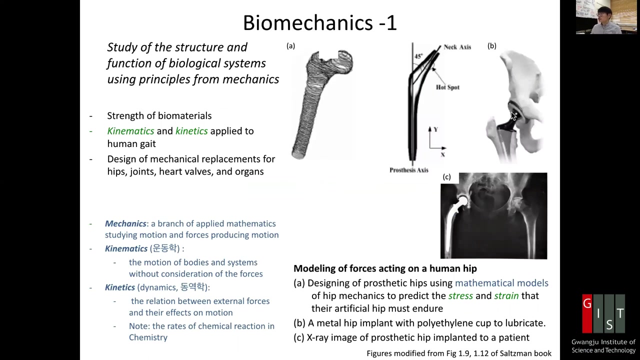 cardiovascular or respiratory function is very much mechanical too. At the same time we also consider in biological tissues the heat and mass transfer. So let's go back to the basics of biomechanics I mentioned previously, to design this to have a function which will last for years. 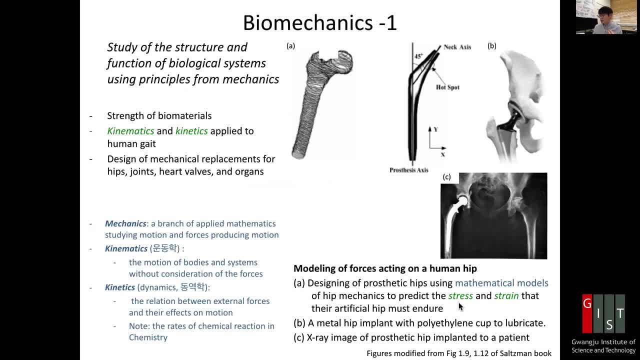 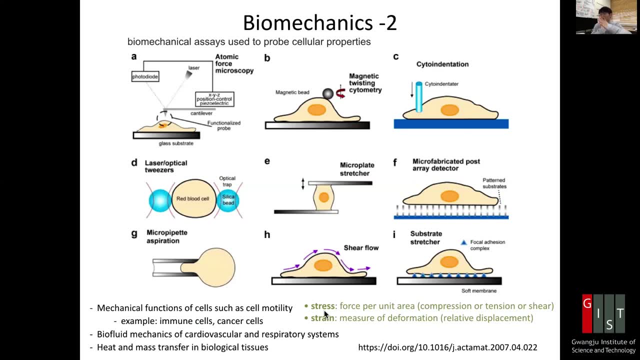 we need to understand the basic stress and strain. So stress is defined as a force per unit area. So, for example, in a compression mode or tensile mode we can compute stress by force per unit area. At the same time all these biomaterials can have a stretch. 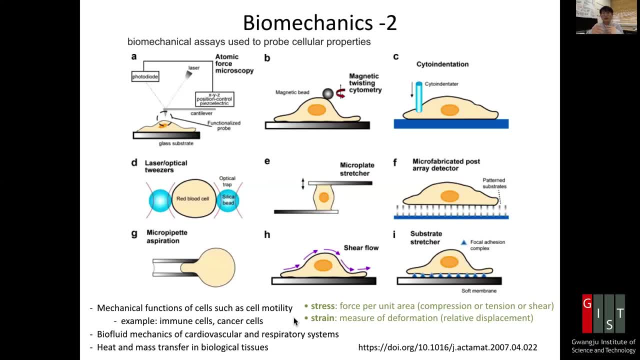 or compression and that will deform. So to define this relative deformation, we can make a definition of measure of deformation which is relative displacement. So strain is defined as the amount of change. So strain is when there is a force, let's say extent. 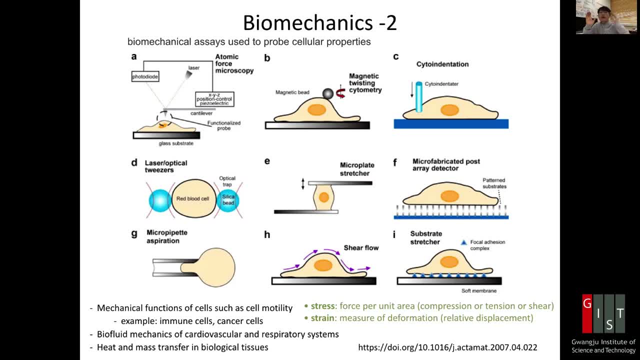 then the amount of displacement divided by its original length, so that it can be normalized in relative displacement. In this interesting chart, which is the exceeds for each, we can apply to平等실 계 eco força. It puts our two watches vertically parallel. 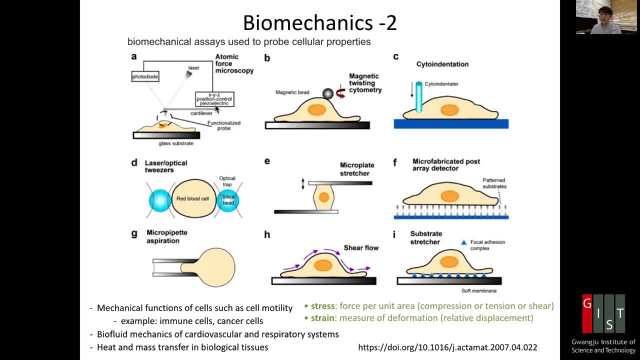 You can see how we can probe a cellular mechanical properties. For example, we can use atomic force microscope to use a cantilever to measure very fine nanometer accuracy. to poke on the cell surface with a functionalized probe to see, to take it away or push, to measure the cellular mechanical property near the cell surface. 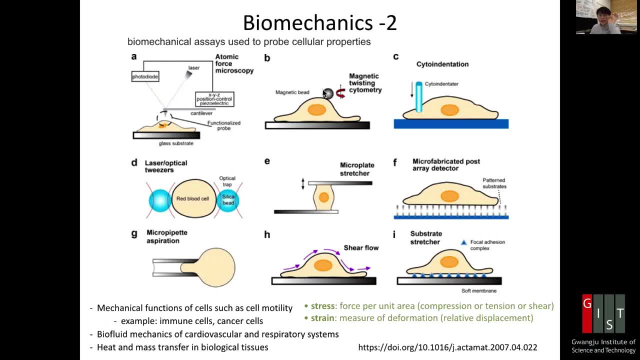 Similarly, we can use magnetic bead to code to attach on a cell, and this magnetic bead you can use external magnetic field to twist and then how the cellular mechanical response to be measured And also cyto-intentation, which is cytomine cell indent, is you're poking the cell and then you can measure the cell's mechanical property. 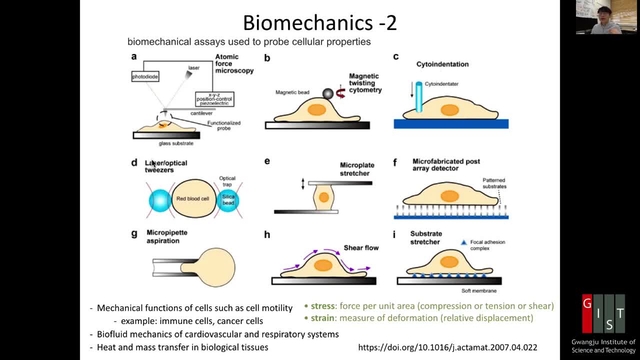 Another fancy way is the so-called laser or optical tweezers, which requires a laser light to focus down and through a silica bead and these optical intensity gradient you can grab a silica bead which is attached to, for example, red blood cell. you can stretch the red blood cell with a defined force and then measure the displacement. 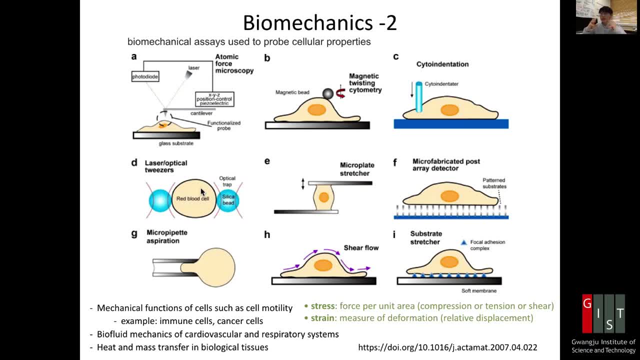 And the second way is the so-called laser or optical tweezers, which gives the mechanical property of the red blood cell Or E. you can see this micro plate stretcher which attach the cell on the other side and then you can exert a defined force and you can measure the displacement. 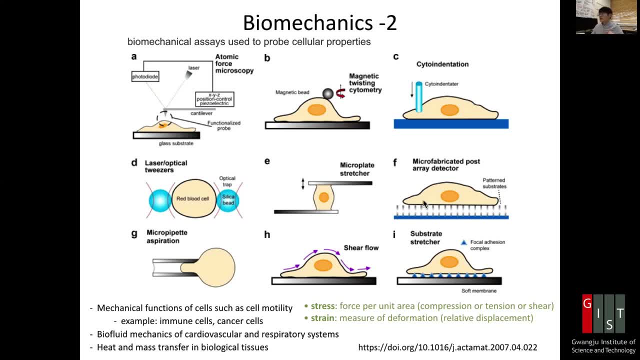 And F. this is using a microfabricated post array detector So you can see the cells are sitting on top of this killer post, Which we know exactly the mechanical property. So this is a patterned surface And you can see from the top view. when the cells move or spread, they exert forces their bottom, which is these posts. 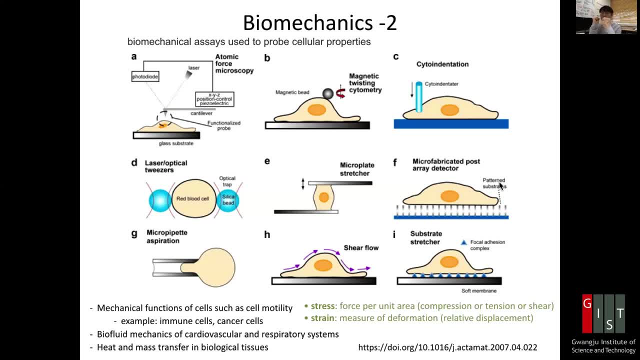 And you can see the post's movement and displacement from the wide field of view. Then you can compute which part of the cell bottoms are actually exposed And you can even compute the amount of force exerted, because you know the mechanical property of this post. microfabricated post. 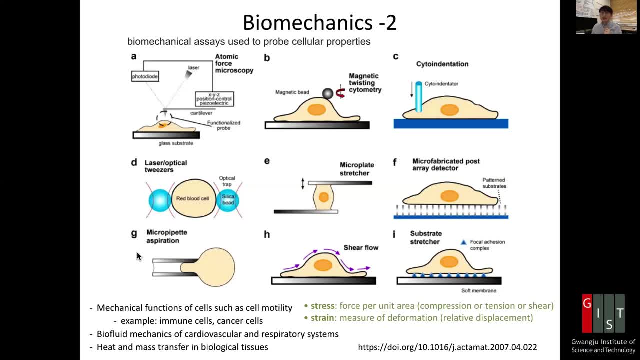 And then G. you may have seen something like this, an in vitro fertilization, a movie. So this is called micropipette aspiration And this is a cell, and you can have a tiny micropipette And let's assume that you can suck it. 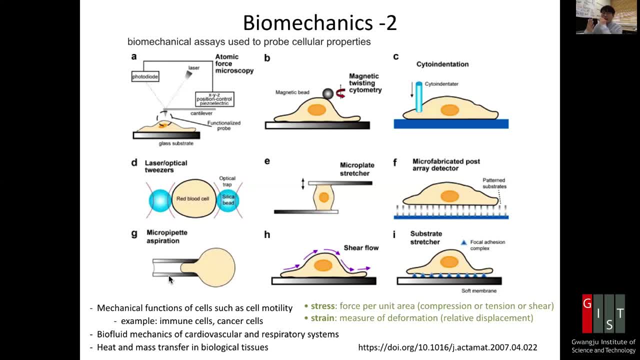 Then if you have you know how much of pressure, of suction force and you can measure the displacement of cell membrane to be inserted, Then you could compute how well the mechanical, the cell stretching property And H you can see on top of a substrate, the cell, you can see shear flow. 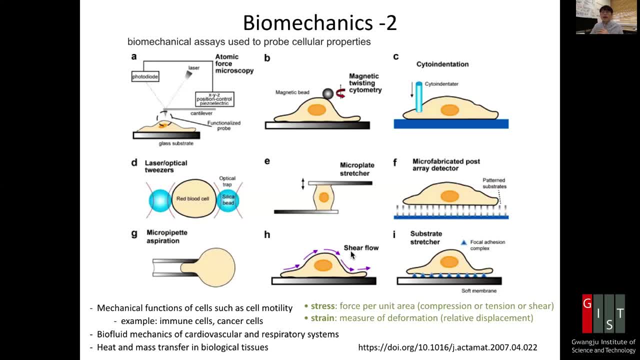 And this might be very important for studying. This is the endothelial cells, which is aligning cells inside our blood vessels, Because blood, there's always a flow And the property of the flow and these endothelial cells- interaction- is very important in some disease, such as atherosclerosis. 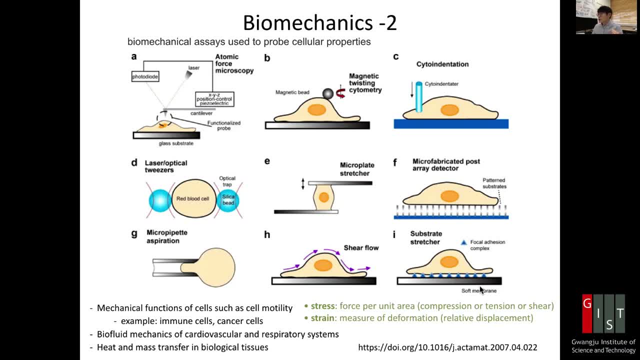 And finally, this substrate structure is: you can use the substrate as a soft membrane And you can label focal adhesives, Focal adhesion complex, which is like a foot process of a cell, And you can label it, in this case with a blue. 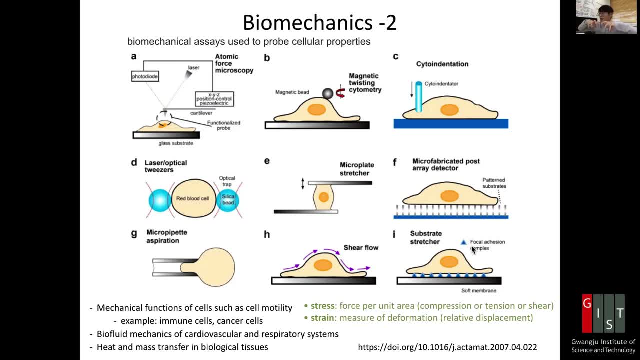 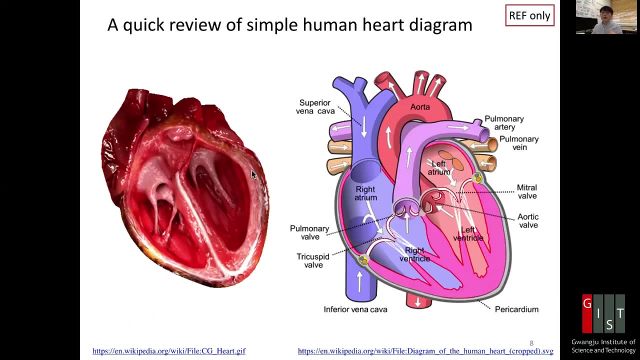 And you can use imaging when the how the cell exert forces to the soft membrane to compute and understand the cell's force on its substrate. This is a reference, but we will talk about heart, So I want to show you the heart movement. 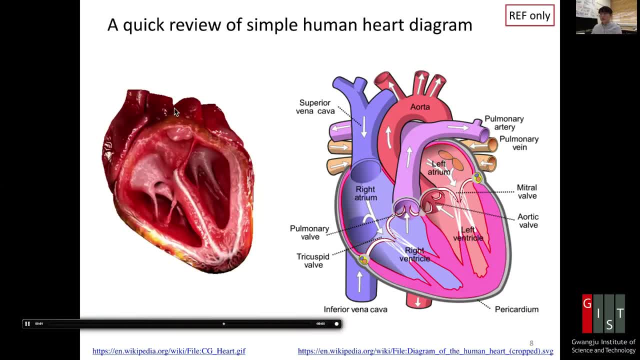 So this is the human heart animation, very realistic, from Wikipedia, And this heart you can see. this is the left part from what we see. However, this is right side of that, So what you are seeing is like humans facing on you. 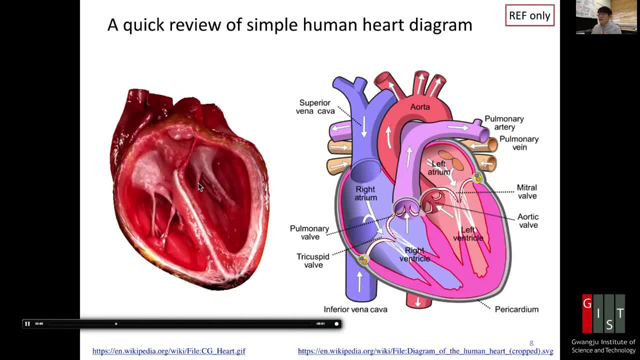 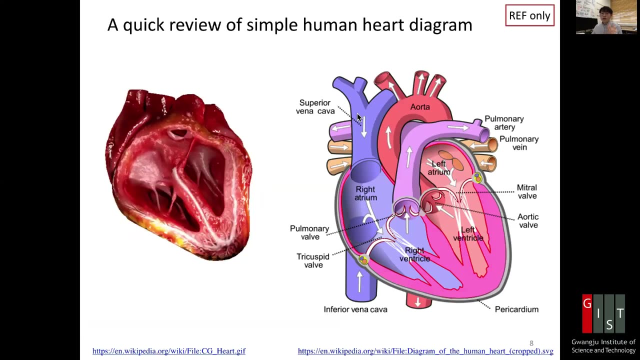 So this is right ventricle, This is left ventricle And on top this floppy part is right atrium And this is left atrium. So most of you probably know, but in a quick summary. So our body, the used body which consumes oxygen and nutrients, will come into right atrium via superior or inferior vena cava. 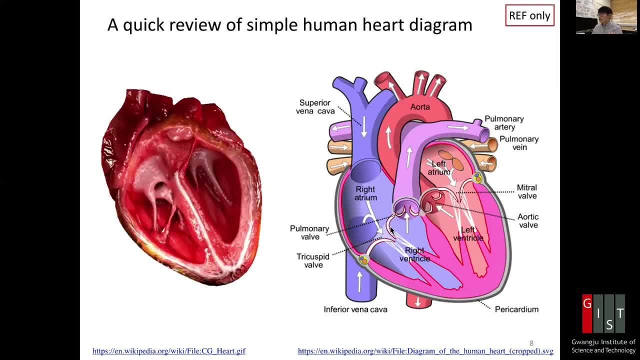 And that blood will pass through this valve into the right ventricle. This is deoxygenated, So it has to go to the lungs to fill with the new, fresh oxygen and exchange it to CO2 content. So it has to go to lungs, sorry, to the, it's called pulmonary artery. 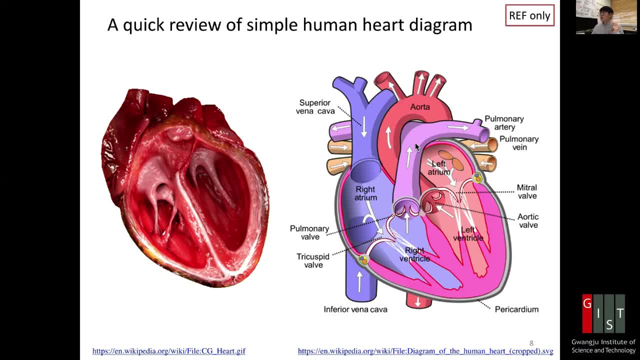 Because pulmonary means lungs, So the important thing is from the heart. when the blood comes from the heart to outside, we name it as an artery, While this is deoxygenated blood, So it can go to right side of the lung, left side of the lung, 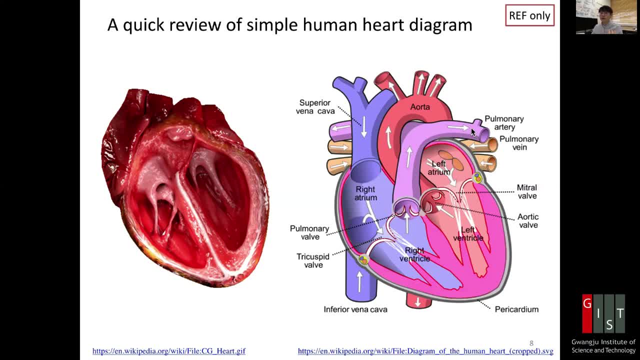 And once it replenishes with a new oxygen, then it can come back to the heart through the pulmonary vein And it goes to left atrium And through this valve it goes to left ventricle. You can see, left ventricle has the biggest and thickest wall, which means it is the pump in our body. 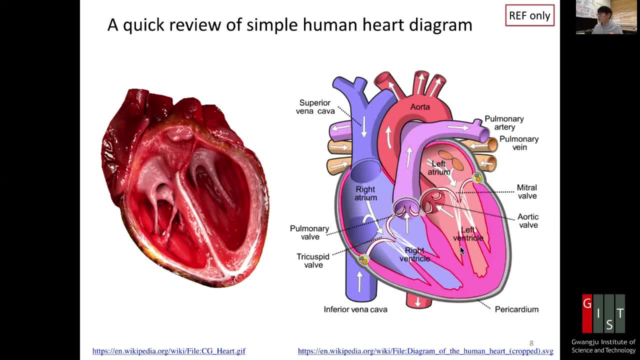 So through that pump of left ventricle it goes, pushing the blood throughout the body. So you can see it is aorta And aortic arch allows the blood goes to upper body and down throughout the body, down. So you can watch this and you can notice the sequence of the valve opening because of this fluid. 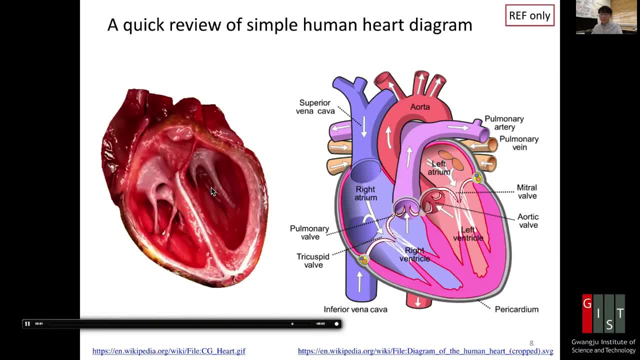 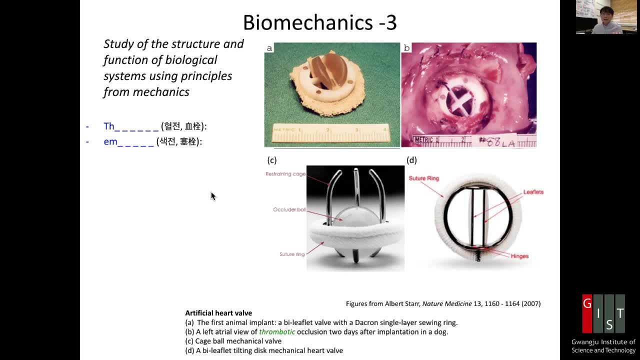 So you can see the flow and direction. Now I want to talk a little more about the disease aspects of the heart. That valve can become a disease and problem for some people. So this is an example of a valve replacement. So this is called artificial heart valve. 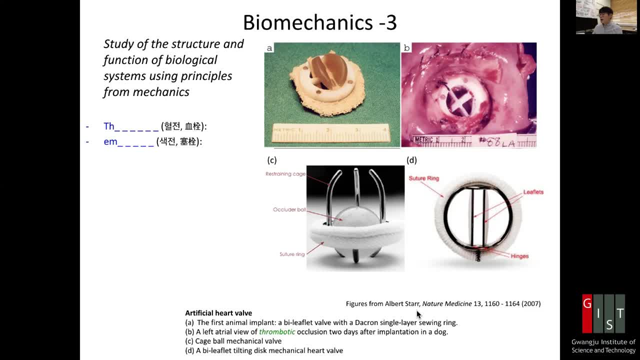 And this is coming from this article. So the A is the first animal implant. So throughout the medical history the suffering person with a heart valve problem, he or she may need a new heart valve. So our human, especially Albert Starr, started animal implant trial. 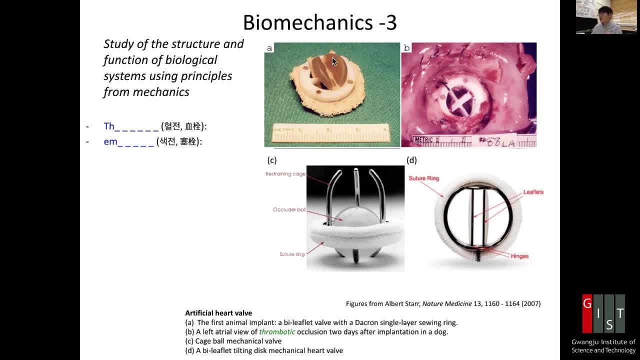 So he developed this bi-liflet. You can see these two liflets- valve with a Declan single layer sewing ring So that you can suture into the existing heart, And he actually put it into implant in a dog. two days after there was a problem in the dog's heart. 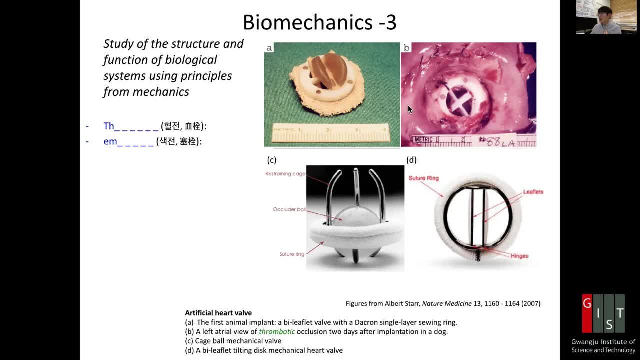 So he took out this heart and examined what happened. So this is left atrial view of thrombotic occlusion And I have to explain you what is thrombotic occlusion. And here is a thrombosis. It means a blood clot formed in here. 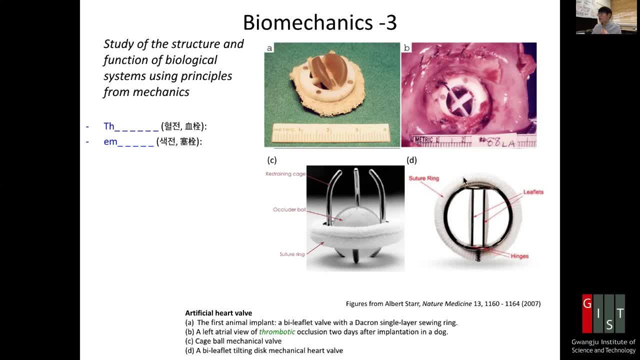 You can see some of the dark ones over here- And that clot occludes, blocks this valve so that the function of the heart will be compromised. So he come up with. since then, humans come up with various ways of better design. One of the design of this artificial heart valve is called cage-bore mechanical valve. 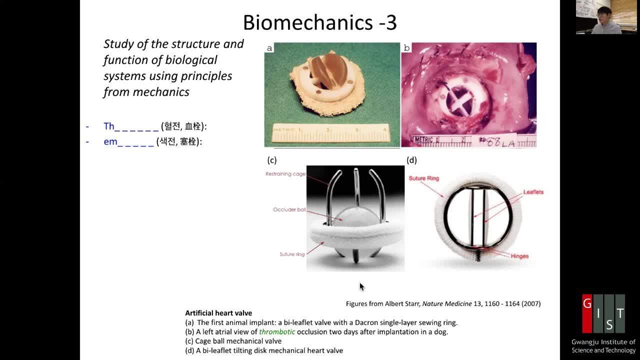 You can even understand from here This bore: when the flow goes from down this direction, the bore is displaced and flow can go. But in the other direction, when the flow try to go back, this bore will block, So function as a valve. 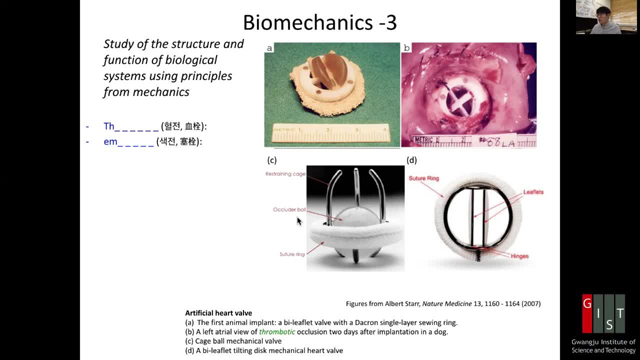 So this wrist training cage, occluder, bore and suture ring serves as a kind of mechanical valve. There's also even another kind. It's bi-liflet. This bi-liflet tilting disc mechanical heart valve. This may make a sound, but in general this heart valve can last years. nowadays, 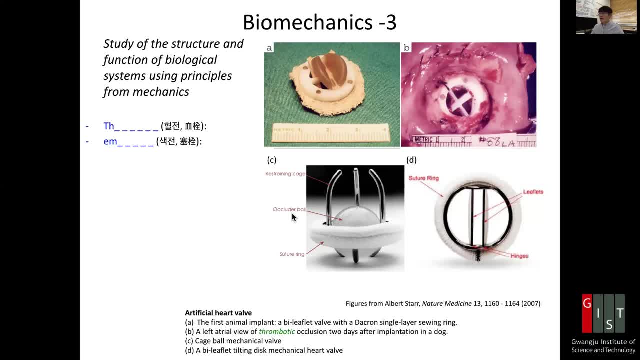 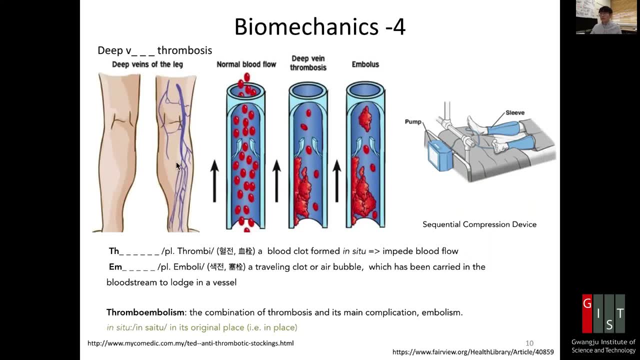 So we have developed this artificial heart quite much Regarding to this blood clot. I want to explain you about this phenomenon of blood clotting, So a medical condition If someone has a surgery and lying down in a patient bag for a very long time. 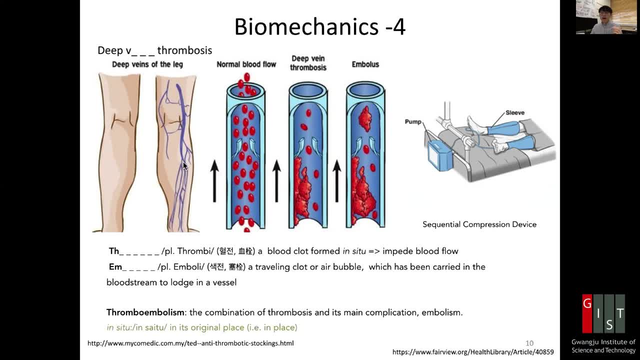 Or some people who have to sit down for hours and hours to a long distance travel. He or she may get in trouble if the blood, if the blood doesn't flow, it is likely to clot, So that is a problem. You can see deep veins of the leg. 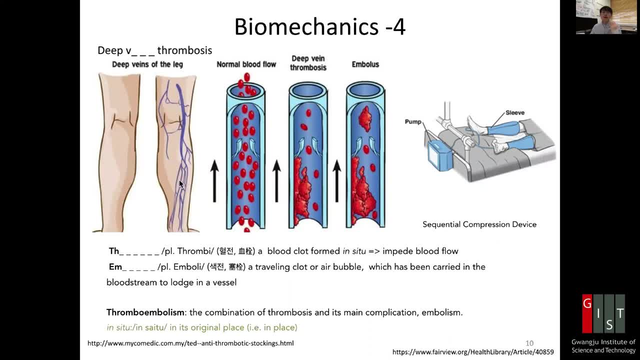 The veins do not have a lot of pressure difference to force the blood to push. Because of that, the veins usually have this valve, which allows the direction of blood flow, only one direction. However, if this is compressed and not moved for a long time, there's a potential that the blood will clot in that location. 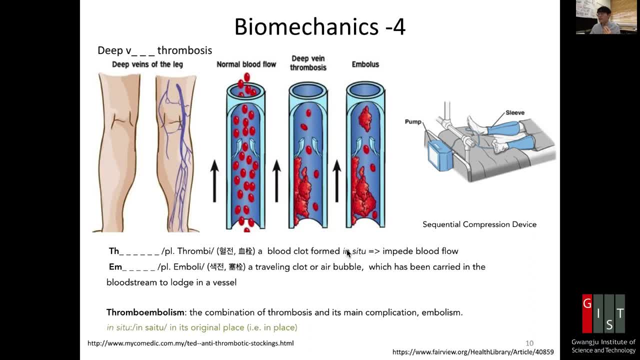 That blood clotting formed in situ. In situ means in its original place, So a local blood clot formed is called a thrombus. So the same plural form is thrombi. So this I becomes US: A thrombus is called this.